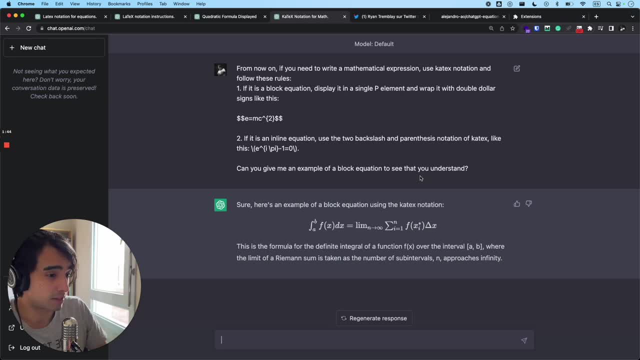 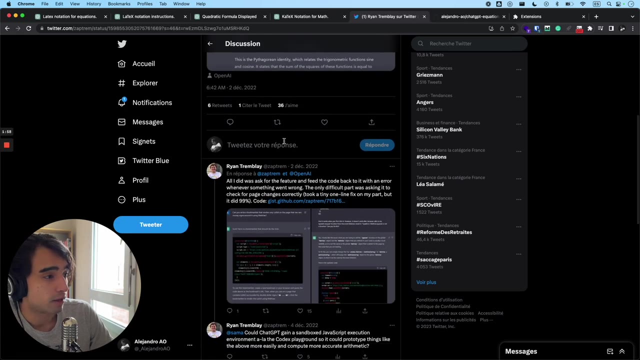 to to print the equation and then go to a LaTeX converter to actually display the equation with beautiful symbols. So basically, I started looking for it. so this is a moment to give a shout-out to this awesome dude who did this pretty much for free and who gave it away for everyone. 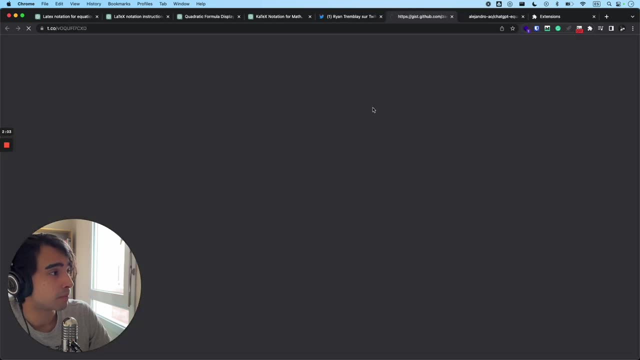 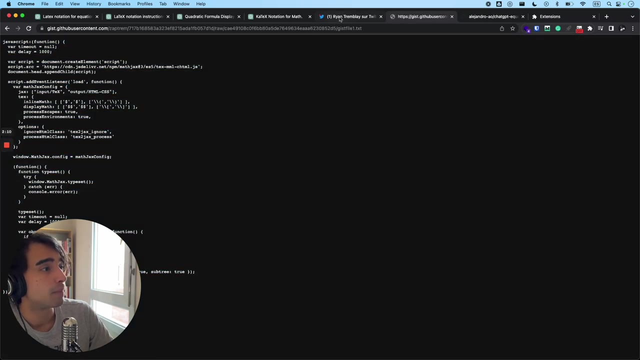 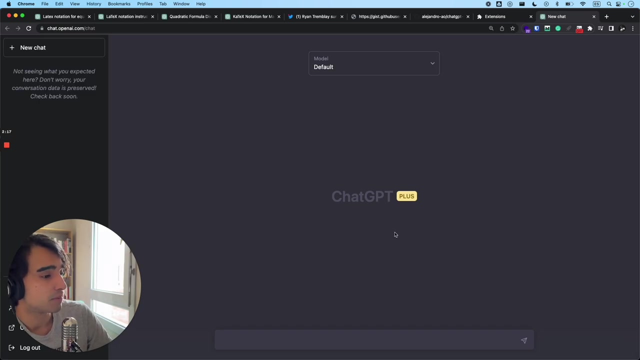 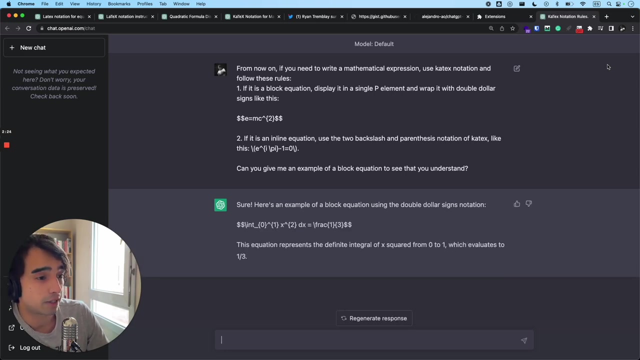 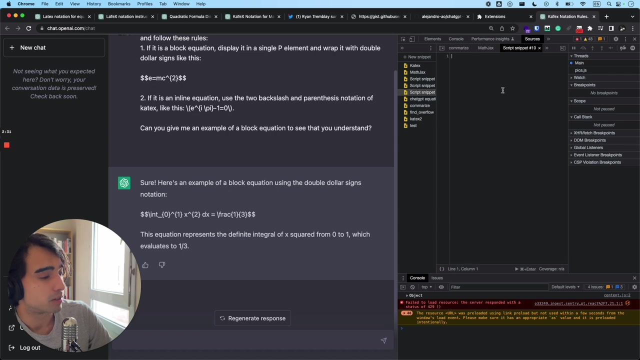 He basically developed exactly what I'm showing you, which is this piece of code right here which you can copy and paste. Paste somewhere where you're using ChatGPT and then just ask ChatGPT to use LaTeX to display mathematical equations, and then you just gotta paste whatever the code he developed and then just hit enter and it's basically going to render the code in ChatGPT. 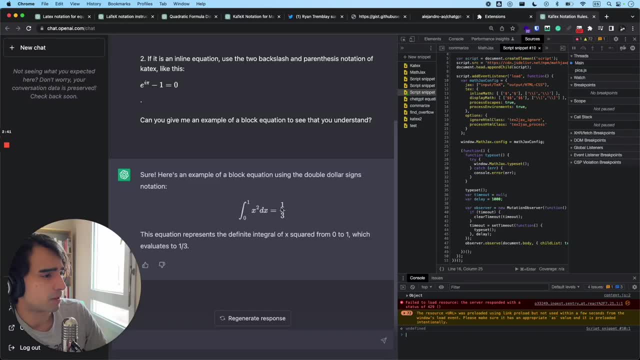 However, I found that there is a problem with this one cause because because If you're using it for a long time, it tends to break. The thing, I suppose, is that either Chrome or ChatGPT doesn't really like having external JavaScript injected in a script tag. 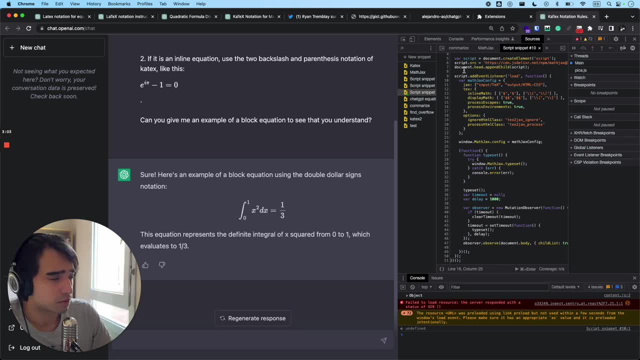 So yeah, after a few minutes it would just crash and I would have to reload, And it was not an extremely good experience. So what I did was basically I just bundled that and repackaged it into this equation right here, which basically does the same thing. 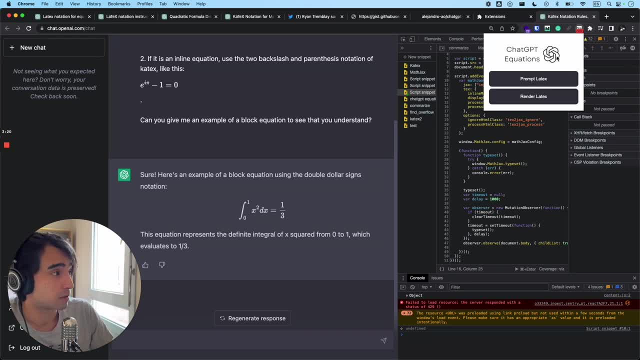 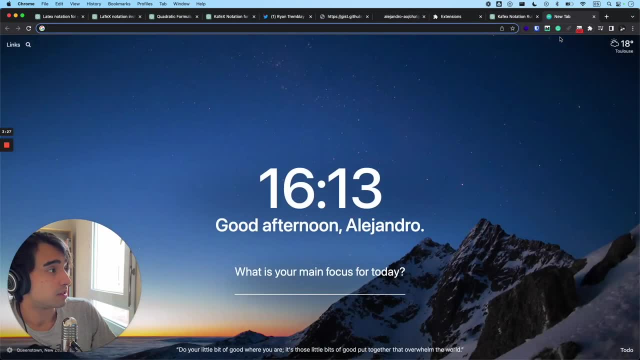 But I've been using it for a few weeks now and it works pretty good, So I'll be showing you how to install it yourself. So, basically, the idea behind the equation is that you go to ChatGPT and you're going to want to ask ChatGPT to display all of the equations using LaTeX. 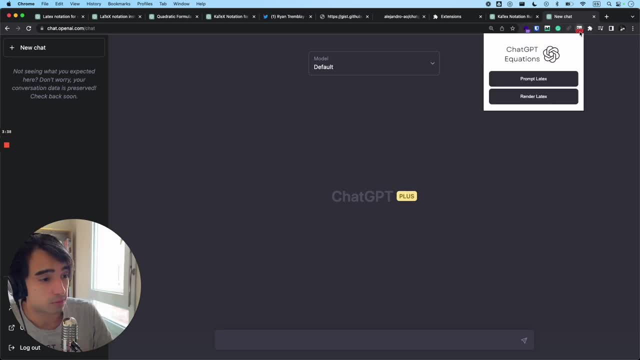 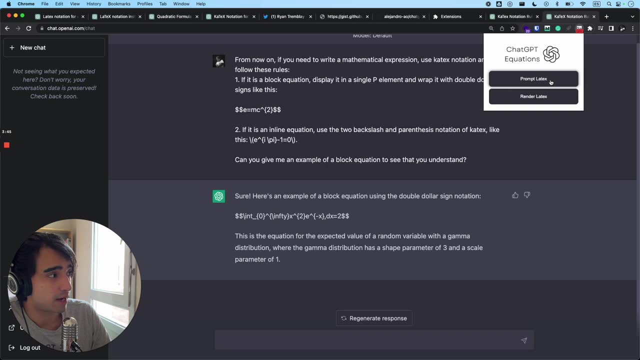 So basically, I mean, what I would do usually is just write a prompt myself, But here I just added a button to ask to create the prompt automatically, And then you have to click on Render LaTeX right, And this basically just takes all of the instances where there is this kind of LaTeX language in the screen. 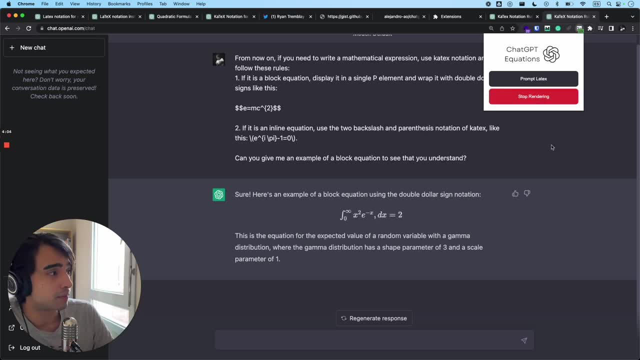 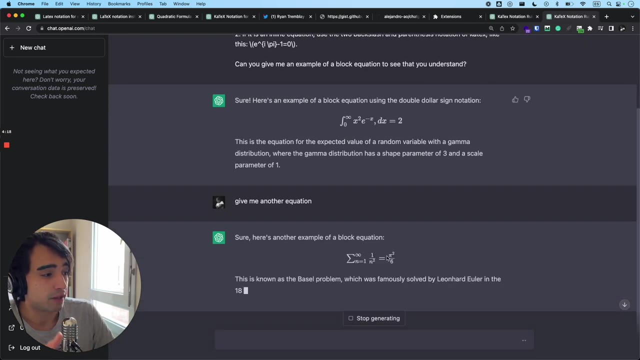 And then it just renders it especially for ChatGPT, right, And then you can just stop the rendering. But the thing is that if you, If you continue working with this- like, for example, give me another equation- It's going to continue rendering it, even if you don't like, press the button again. 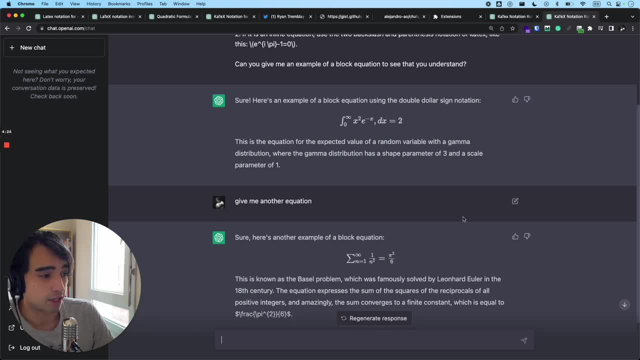 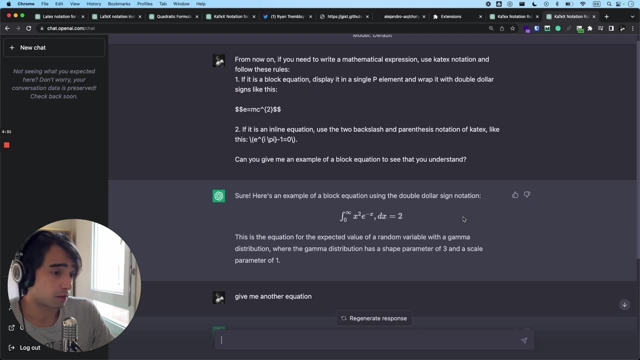 It's like continuously rendering every LaTeX expression in the screen. So I mean that part is pretty useful. For the moment it only works on ChatGPT, because that's where I was using it, And so now I'm going to show you how to install it. 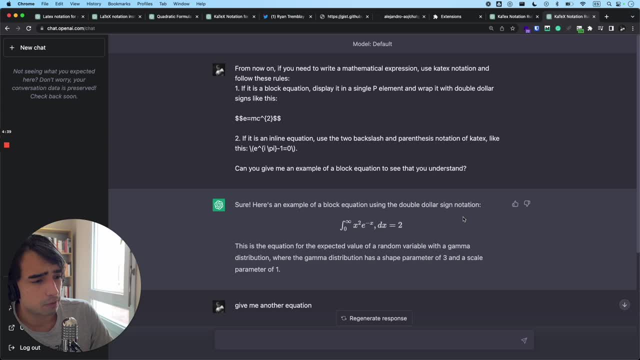 To install it. I actually tried To put it on Chrome Web Store this weekend, But it's taken a bit of time to actually have it like, go through all the permissions and like to have it validated. So I'm going to show you how to install it from GitHub. 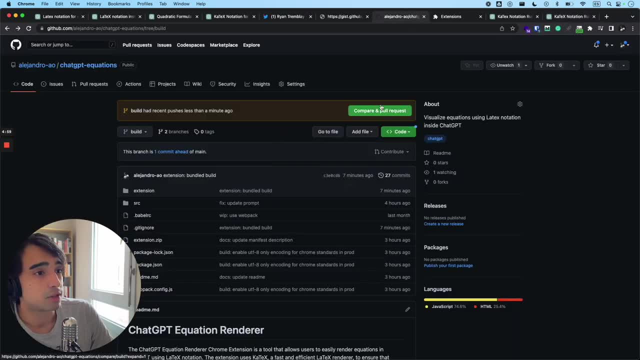 So I'm going to put this link in the description, which is a link to the repository of the extension And, of course, if you're a developer, you can totally contribute to it And just send a pull request and we can go through it. 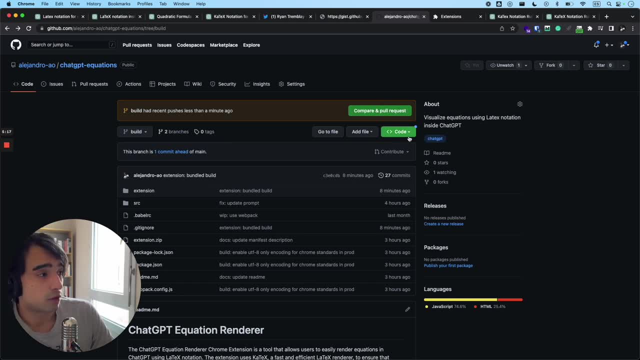 But the idea here is that if you want to install it in your computer, you're going to want to come here- I mean to go to the link in the description- And then you're going to come here to code And then click on download. zip right. 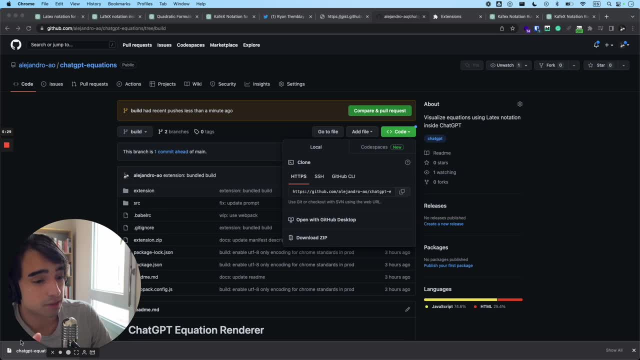 That'll download this file right here. You will have to unzip it Like. like in Mac, you can just unzip it by clicking on it like this, And here you have it All right, So inside the file. let me show you what it looks like. 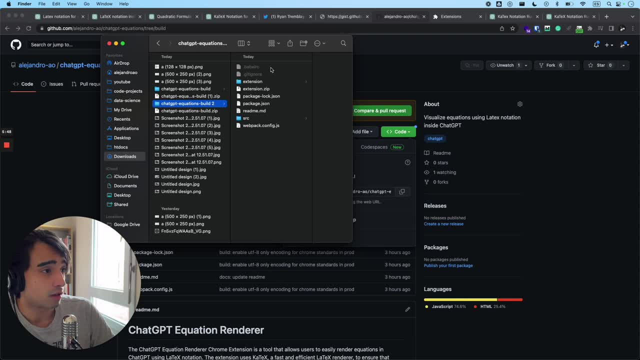 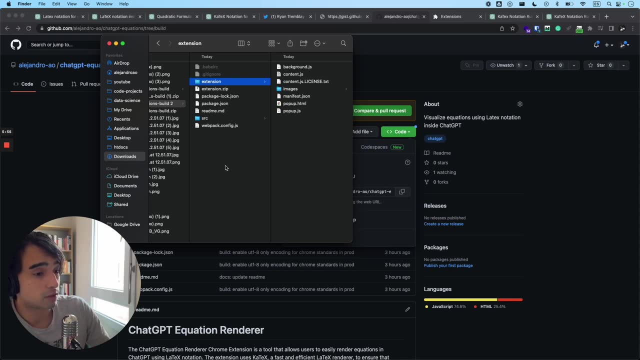 Inside the file, inside the unzipped file, you will have this folder. right here It's called extension. The rest of it is basically just to build it. I mean, if you're a developer, you know what these kind of things are. 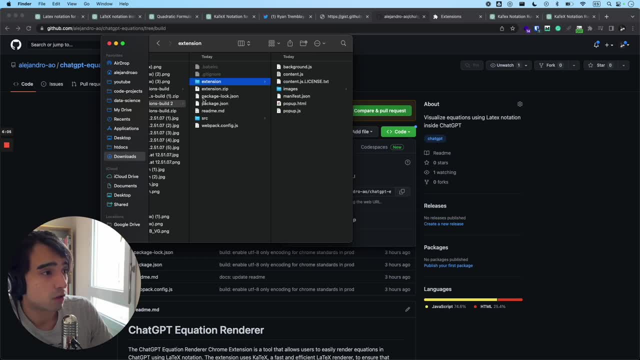 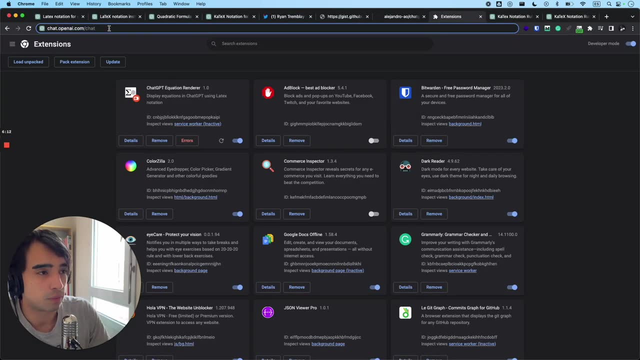 But if you just want to install it in your browser, the only folder that you're interested in is extension, right here. So In order to install it in your browser, you're going to have to go to in your browser. You're going to have to go to Chrome extensions, which is like the list of your extensions that you have installed. 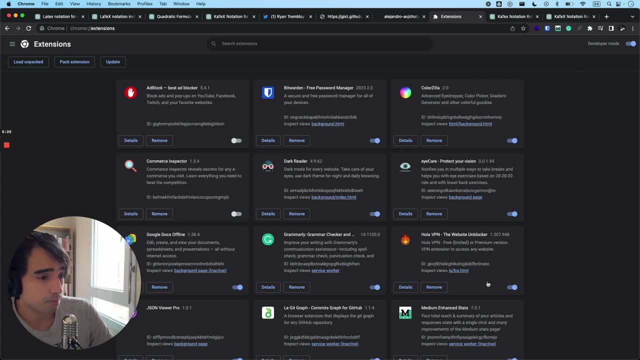 I'm just going to remove the one that I already have here installed And you're going to have to click right here and develop developer mode so that you can see this button right here which is load unpacked. Then you're going to click on load unpacked. 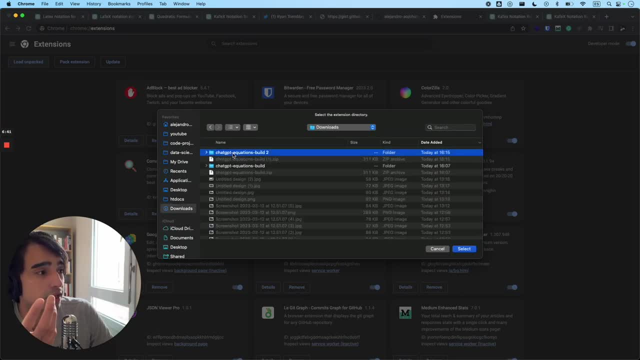 And you're going to have to go to the browser And you're going to look for the extension that you just downloaded Right, And inside the file you're going to select the extension button Right. I mean, ideally, I would place this not in the downloads folder but in some folder that I know that I'm going to keep for a long time, because if you delete this folder, you're going to delete the extension as well. 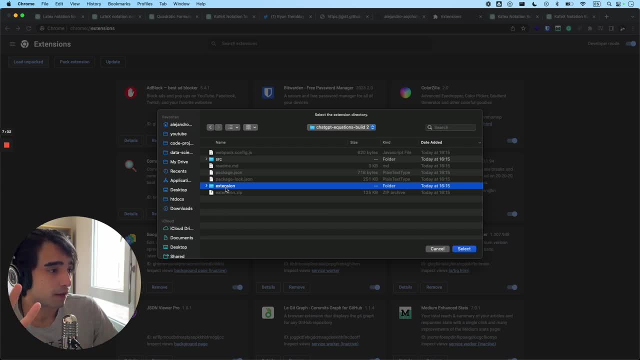 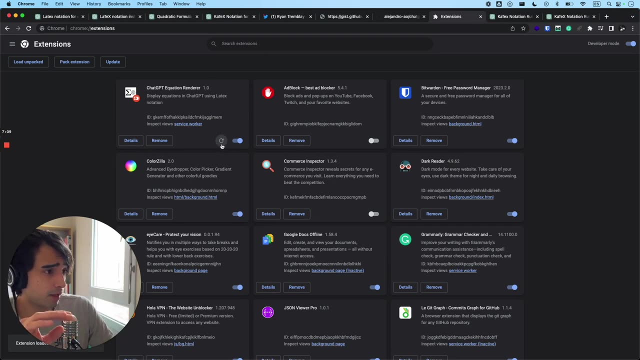 So I would just put it in my documents or wherever you want, and then just select the extension folder. click and select, Then it's going to load it And if, for some reason, the extension crashes, you're just going to have to click right here and refresh the extension. 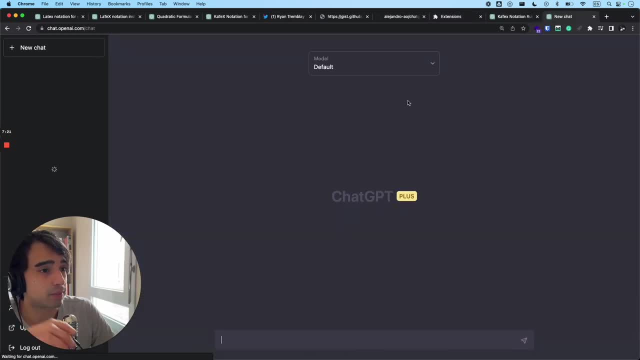 And now you can definitely just go to ChatGPT like this and you will have this new extension right here, which is ChatGPT equation renderer. I chose just to pin it here and then you click on it. You have a pop up, the first button. 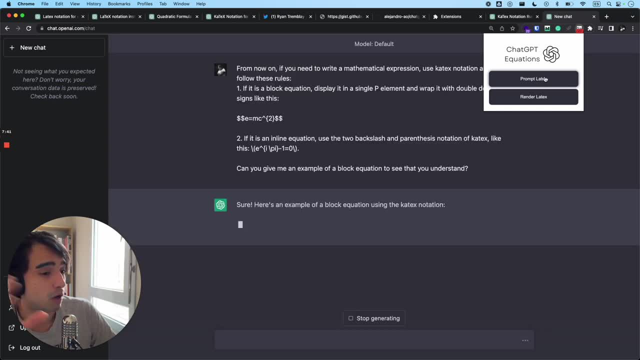 It does what I showed you already. It automatically creates the prompt for ChatGPT and it asks it to use LaTeX to render equations, And then you just render all the equations in its request And, as you can see, the renderer is turning all while you have this enabled. 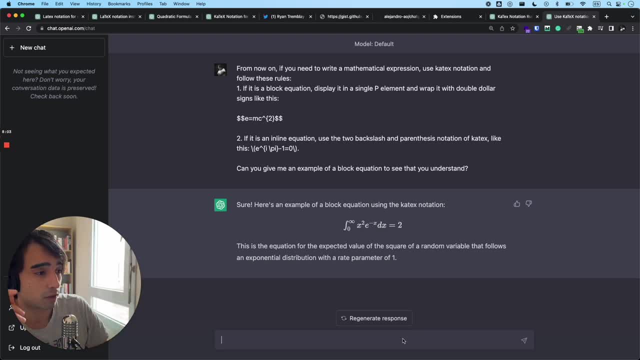 So you can continue asking for I mean, you can just continue your study session and your all of your equations will be Inverted into this beautiful syntax like symbols. So yeah, I mean I'm sure that if someone has done, has a little bit more experience with ChatGPT, maybe there is a prompt to actually do this without an extension. 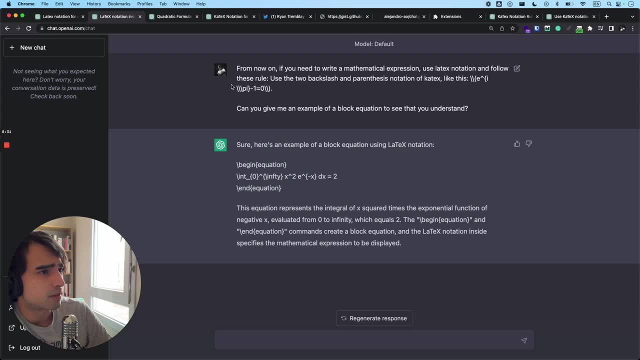 I have been trying to do something like this. These are some tests that I that I used. I mean, at some point it worked to do This and then I made it work And then I just pulled it out. I'm not gonna do it again.